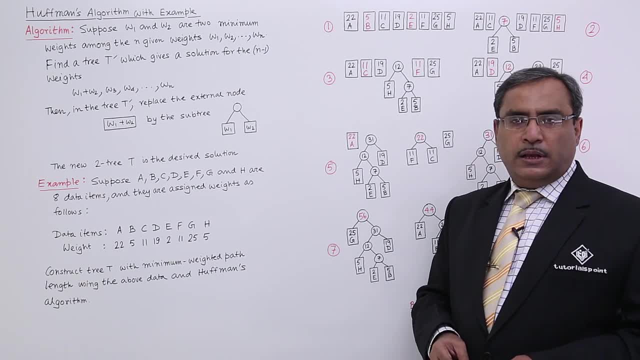 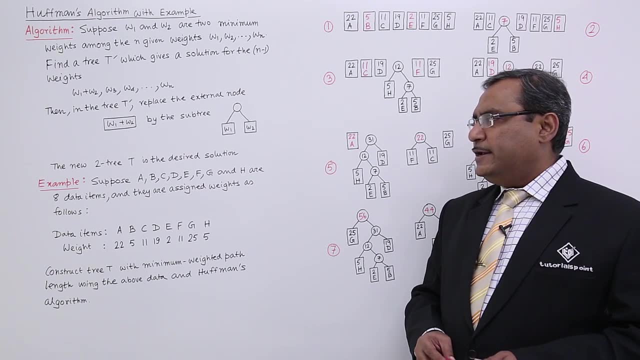 So to get a better understanding on this particular Huffman's algorithm, let us go for one example. Suppose a, b, c, d, e, f, g and h are eight data items and they are assigned weights as follows: Data items are a, b, c, d, e, f, g, h and the respective weights are: 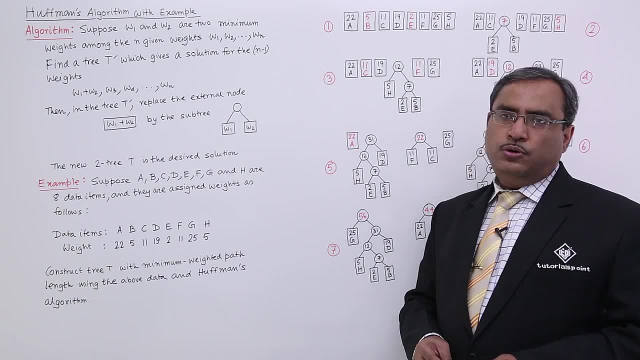 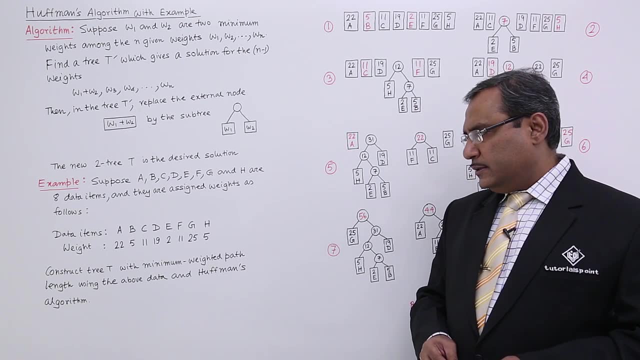 w1, w2,, dot, dot, dot up to wn. find a tree t dash which gives a solution for the n minus 1 point, sum 22,, 5,, 11,, 19,, 2,, 11,, 25 and 5.. Construct tree trees with minimum weighted path. 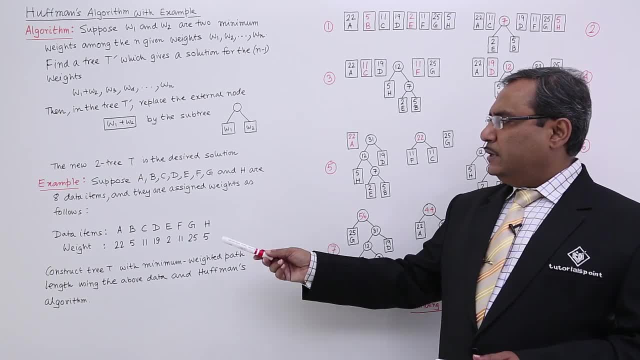 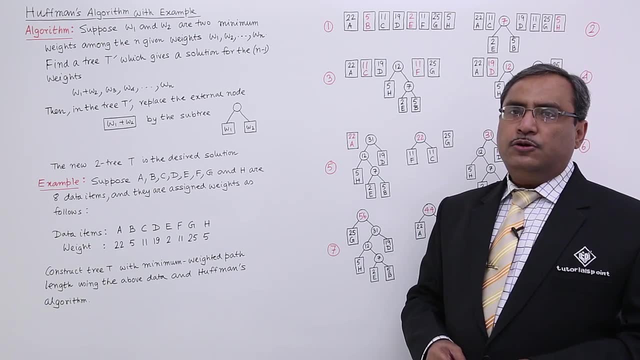 lengths using the above data and the Huffman's algorithm. So this particular above data, on this particular above data, Huffman's algorithm will be applied to generate the external two tree as the solution and there this particular algorithm will be used in a recursive way. 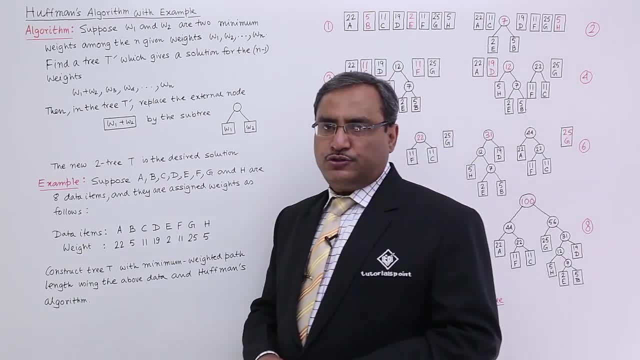 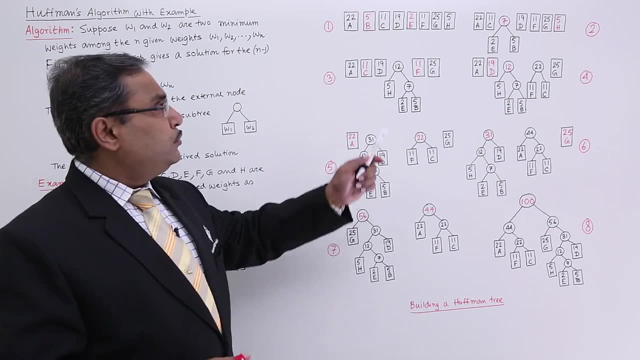 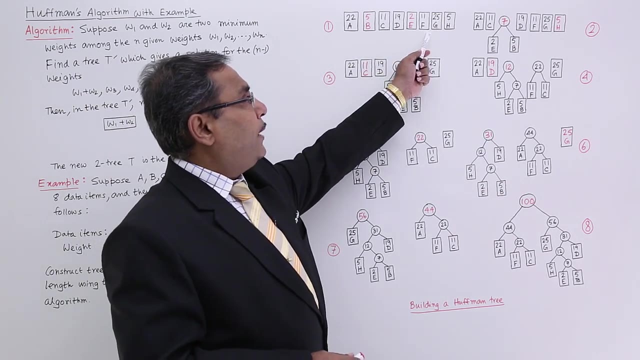 constructed in the bottom map approach. so let us go for the solution. see, so this is my: the respective weight, age and data we have written. now i shall have to select the minimum two nodes having the minimum weights. so here they are: five and two. i could have taken this five also. 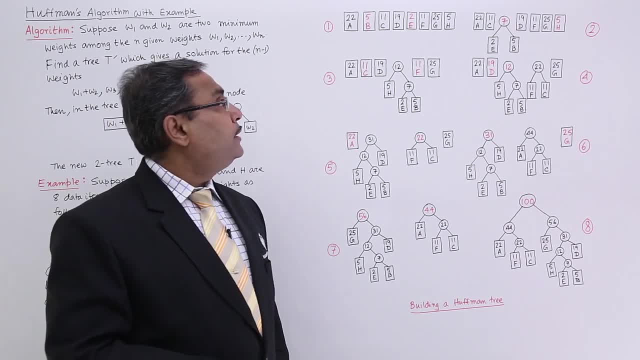 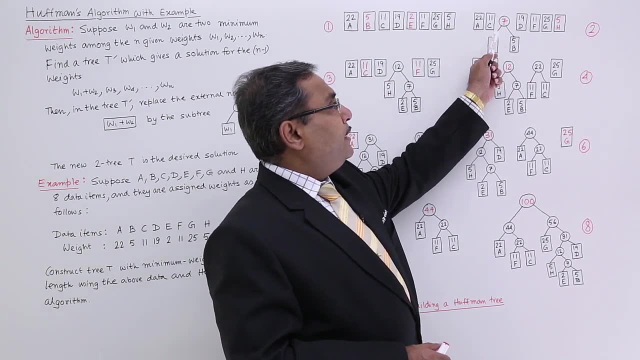 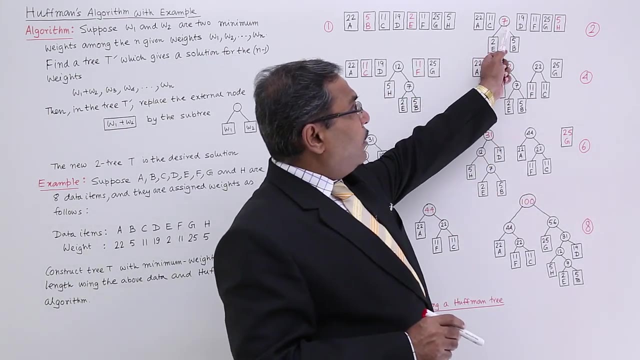 so tie should be broken arbitrarily. so i have taken this five and this two. so now this five and two will be added and i'll be getting seven, and these two are the respective nodes will be there, like this one: okay, so now out. so now this seven will be taken in in the participation. 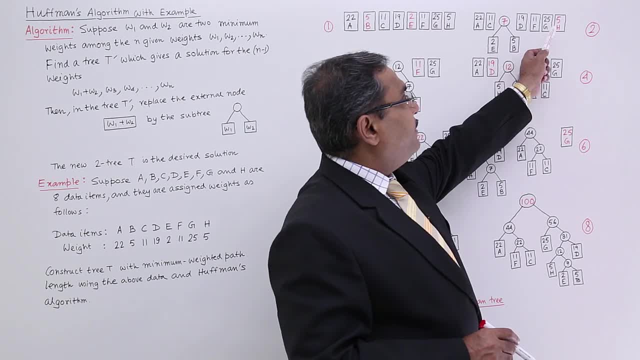 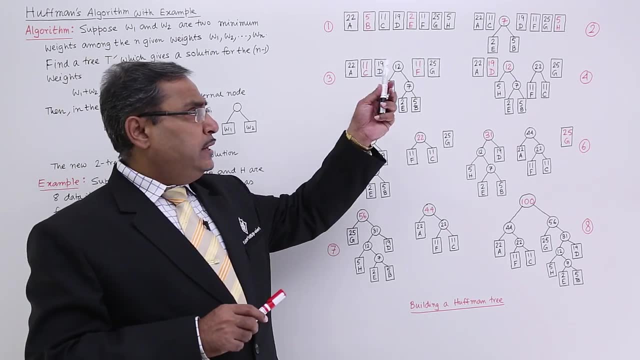 so 22, 11, 7, 19, 11, 25, 5. so out of them i shall have to find out two minimum weight ages. so i'm getting seven and five. intentionally we have colored them with the red, so seven and five will be there. so 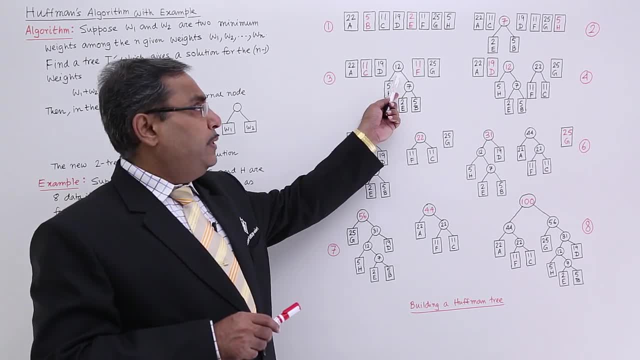 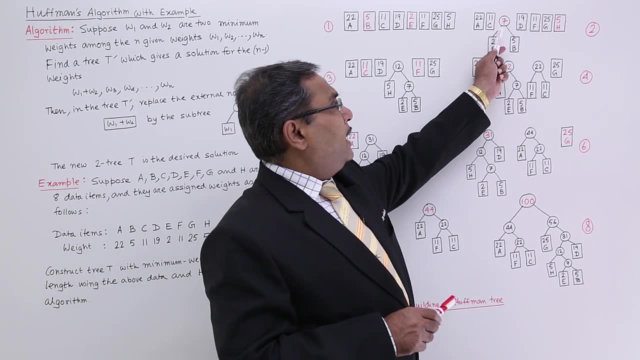 they will form this one. so 12 will be coming. so 12 will be coming. so w1 plus w2 will be the node, so 12 will be coming, and and then obviously it will be as one of the subtree and it will be coming as the one of the one of the left child. or right child. okay, so that is my five h and this seven, this one seven. this one means this one. now, out of this, 22, 11, 19, 12, 11 and 25, i shall have to find out two minimum weights. so here i'm. 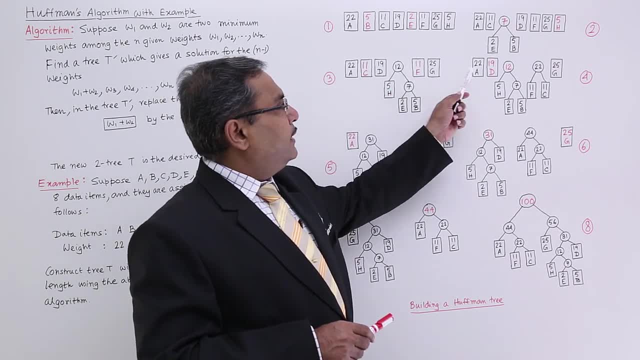 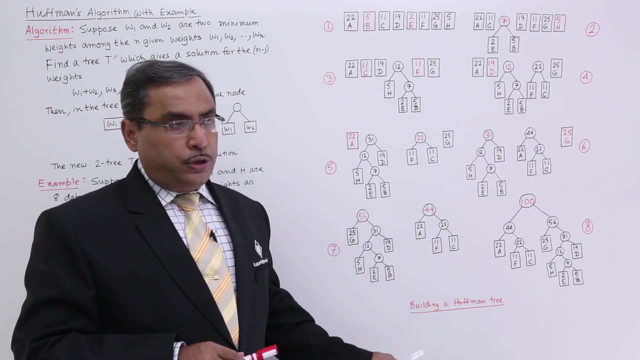 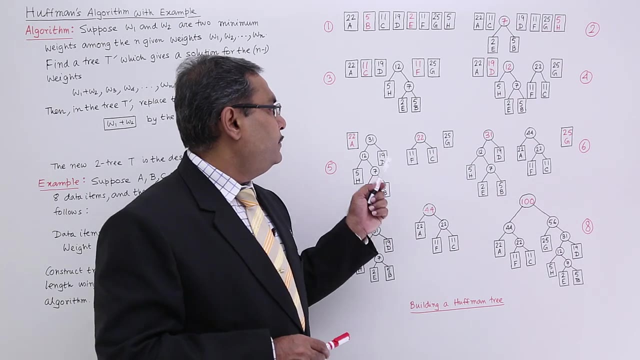 getting 11 and 11. so this 11 and 11 they are. so i'm making this 22 with this 11 and 11. f and c are two children. in this way, the process will be continued. so, out of this, 22, 19, 12, 22 and 25, 19 and 12 are the minimum. so i'm forming this. 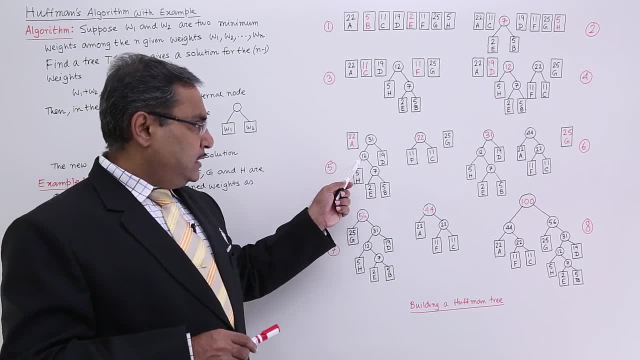 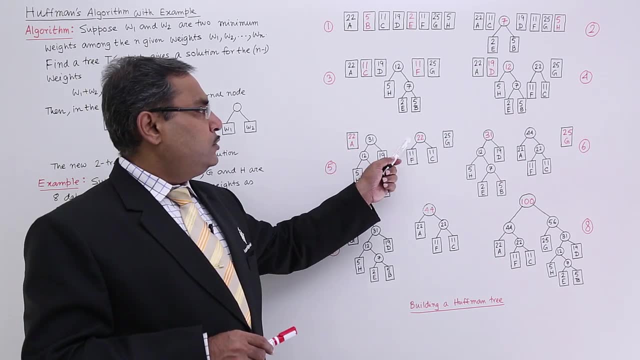 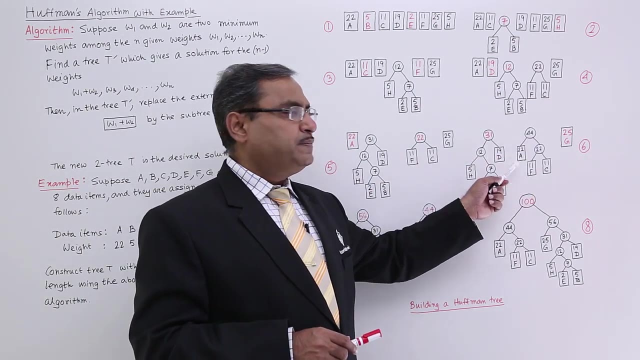 31, adding w1 plus w2 and this and there and others have got the respective sub trees okay. so 22, 31, 22 and 25, out of them 222 the minimum. so i'm forming this 44 and this particular tree, and then 31 and 25 will be. 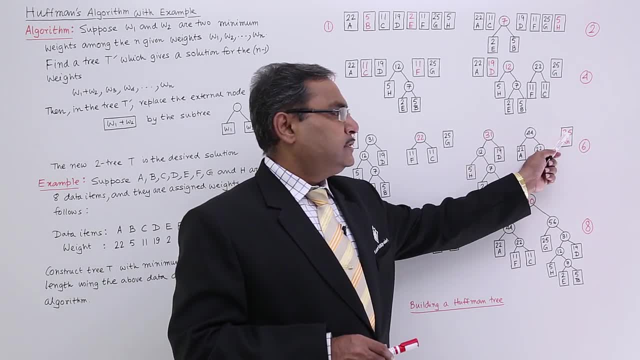 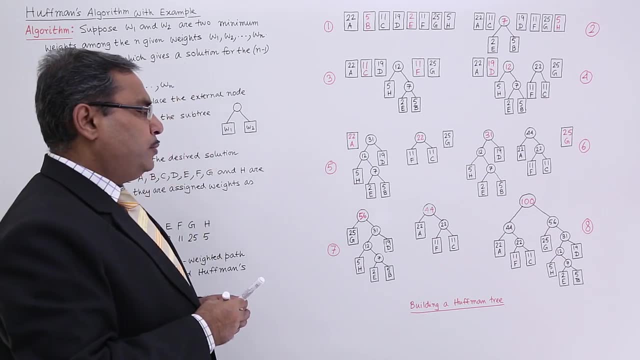 minimum out of this three, so 35 plus uh, 31 plus 25, it will become 56. so 56 will be coming down here. so 56 will be coming down here and we are having this others as a sub trees. so now we are having 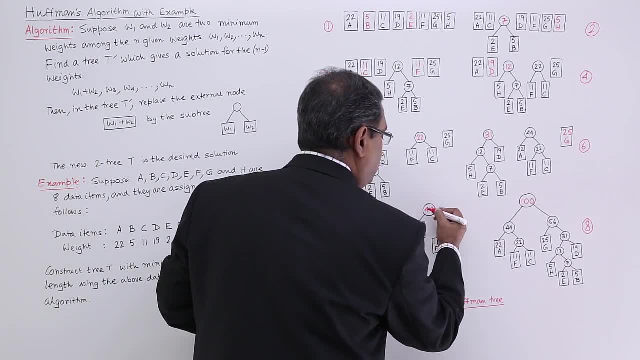 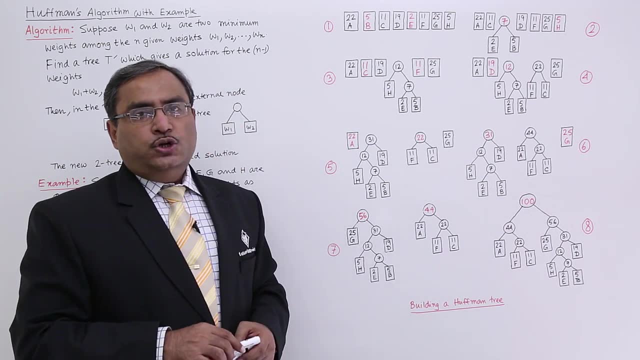 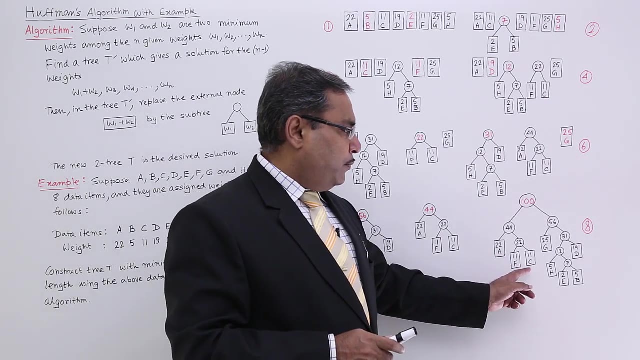 this 44 and 56, so there is no other choice because only two data items are remaining. so 44 and 56, so they'll be coming as a hundred and in this way, this two tree, or external binary tree, we have formed this one, you are getting this one- that this rectangular box shaped nodes are the external nodes. 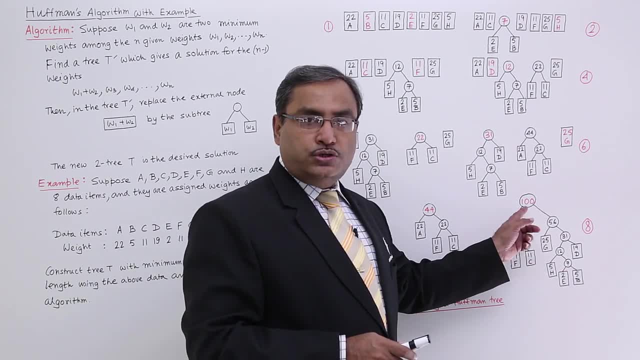 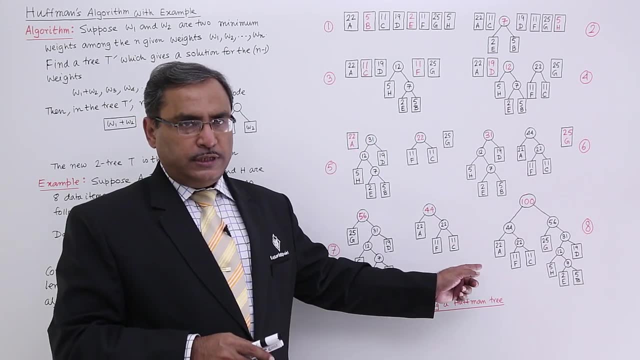 and this circular, circularly enclosed nodes are the internal nodes and it is known as two tree. so in this way you are getting this two tree, which has been formed using this halfman's algorithm, and this tree is also known as halfman tree. so building a halfman tree so that 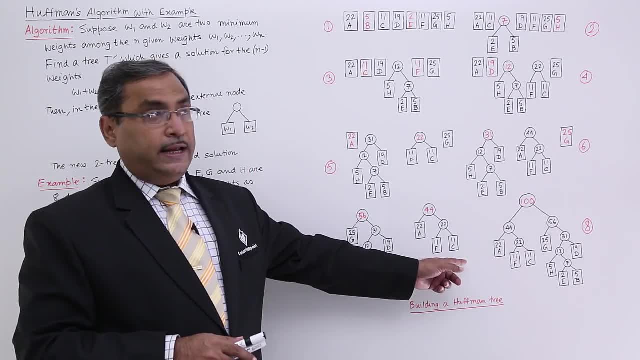 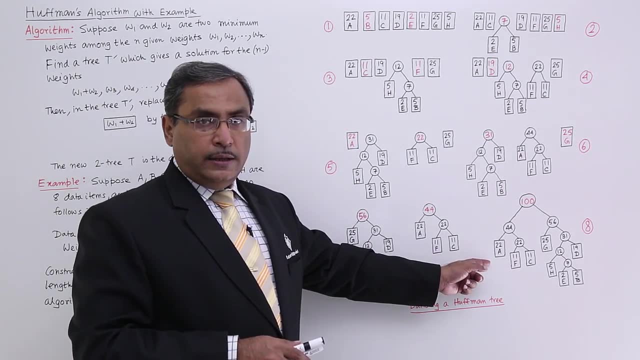 is the halfman tree we have built and that is the solution we are getting. and in this way we have numbered this particular figures. so one, two, three, four up to eight. so in the figure number eight i'm getting, i'm having this particular solution at the eighth figure. so in this way, 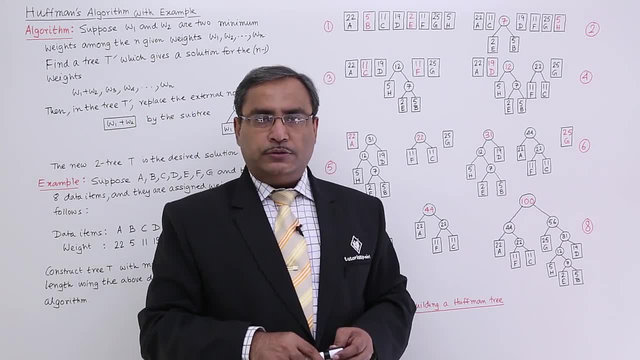 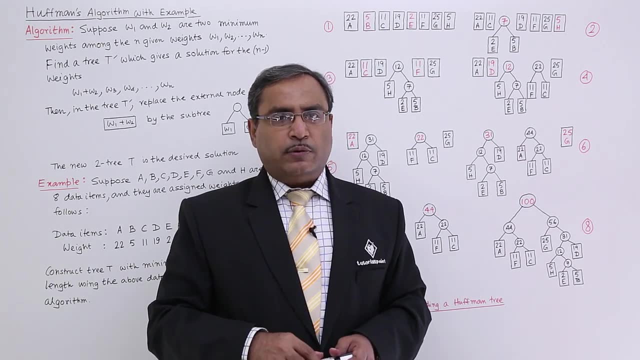 using this halfman algorithm, the halfman tree can be formed. so please do this. do some practice with some other set of data and get a grip over the subject. thanks for watching this video.